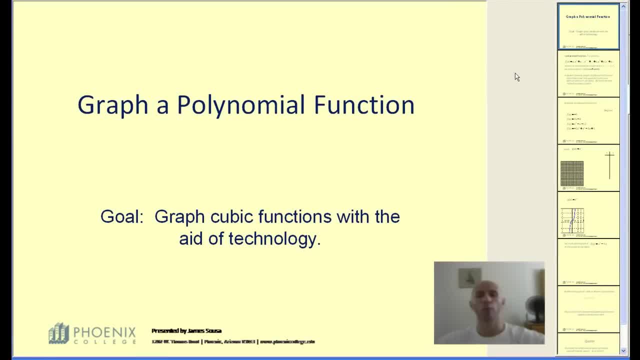 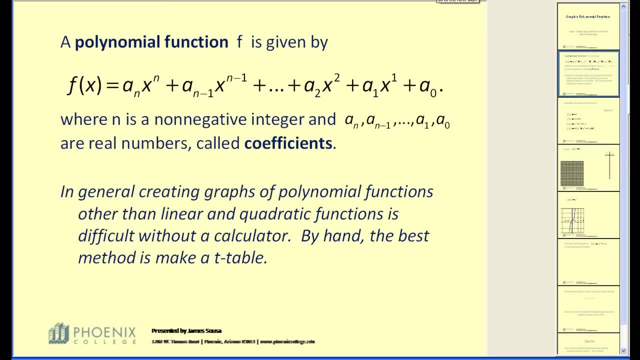 Graph a polynomial function. Our goal, more specifically, is to be able to graph cubic functions with the aid of technology. A polynomial function is a function given in this form. Now, this may look complicated and involved, but in fact, it's not quite as bad as you might be thinking. n or the exponents are just. 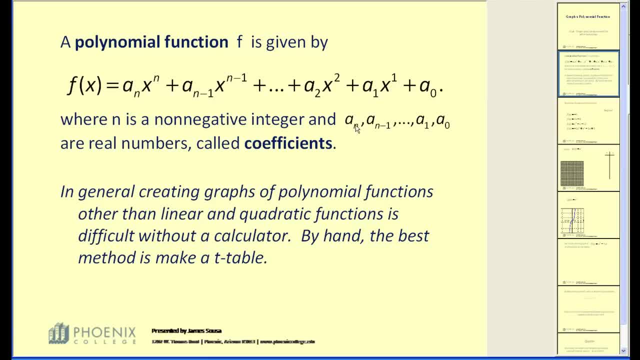 any non-negative integer and the a's with all of these subscripts are just the coefficients and these must be real numbers. In general, creating graphs of polynomial functions other than linear and quadratic functions is difficult without a calculator By hand. the best method is to make a t-table. Let's go. 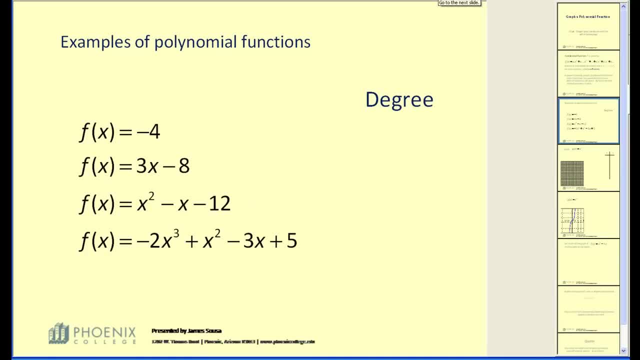 ahead and take a look at some examples of polynomial functions that you're already familiar with. f of x equals negative 4, known as the constant function, and just review, that is a polynomial function of degrees 0.. f of x equals 3x minus 8. of course is a linear function. This is a polynomial. 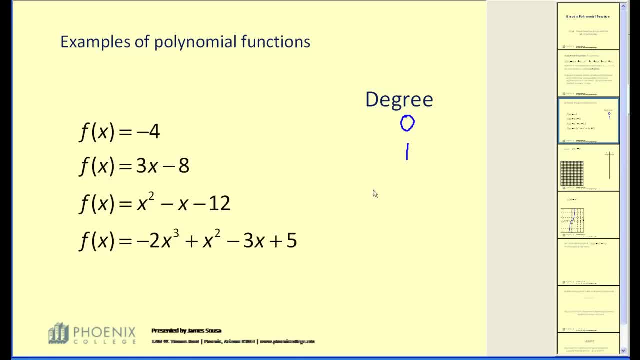 function of degree 1.. The next function f of x equals x squared minus x minus 12.. A quadratic function, also a polynomial function, of degree 2. and then the last function f of x equals negative x cubed plus x squared minus 3x plus 7. That's. 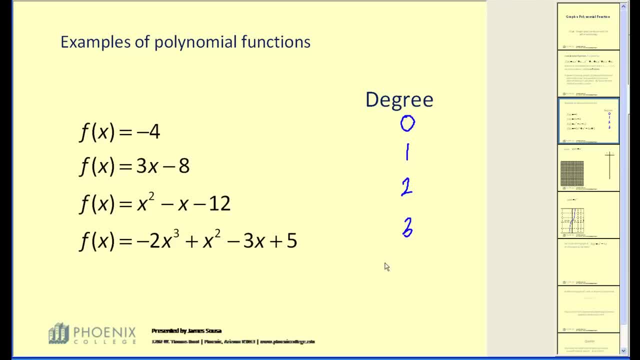 known as a cubic function of degree 3.. Of course we could make higher and higher degree functions here. That would all be polynomial functions. You kind of see the pattern. Let's go and take a look at the graph of one of the most basic polynomial functions and 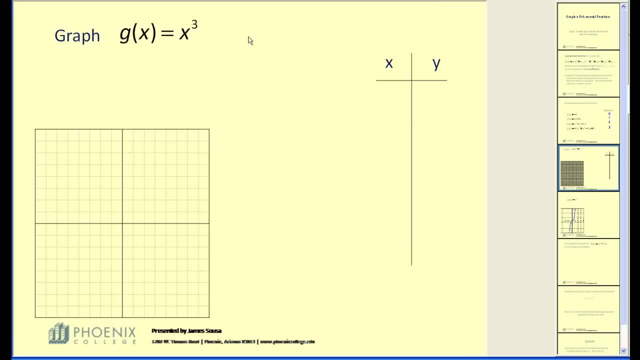 in fact, because it is a degree 3 polynomial function, this is your basic cubic function. Now, if we're not familiar with how to make this graph, it's always a good idea to go back to the t-table. So I'm going to go ahead and pick some x. 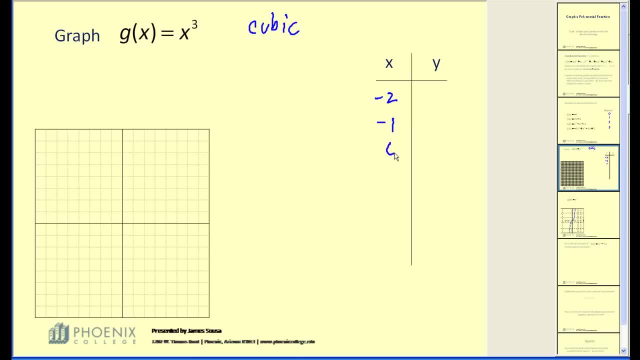 values. Substitute these values into the function and find the corresponding y value. I'll show a couple of these. The first value of x that we chose was negative 2.. f of negative 2 is equal to negative 2 raised to the third power, which of course is: 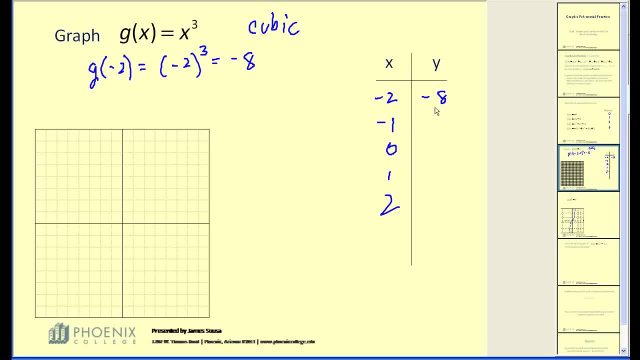 negative 8.. The rest of these you can probably do in our heads. If you cube negative 1, you get negative 1.. Cube 0, 0. If you cube 1 or raise 1 to the third power, you get a. 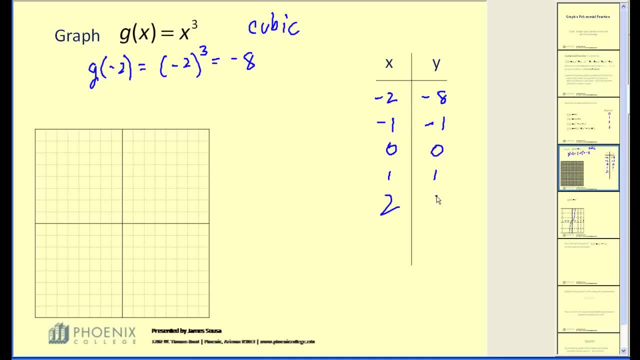 positive 1.. If you raise positive 2 to the third power, you get a positive 1.. Let's go ahead and plot these points and see what we have. If this is not enough points to see what the graph would look like, or if we're not sure we need to, 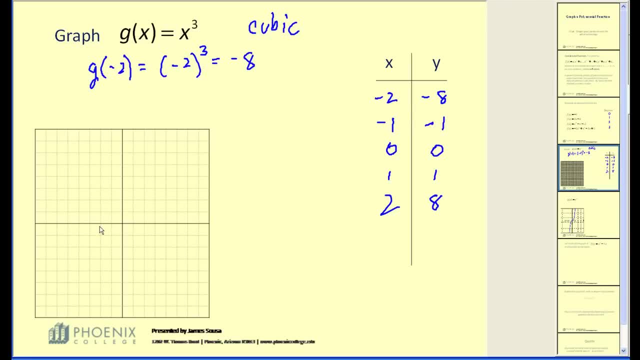 pick some more points: Negative 2, negative 8, negative 1, negative 1, 0, 0, 1, 1, and 2, 8.. Now, this graph does have a curve to it. If we take a look at the graph on with some 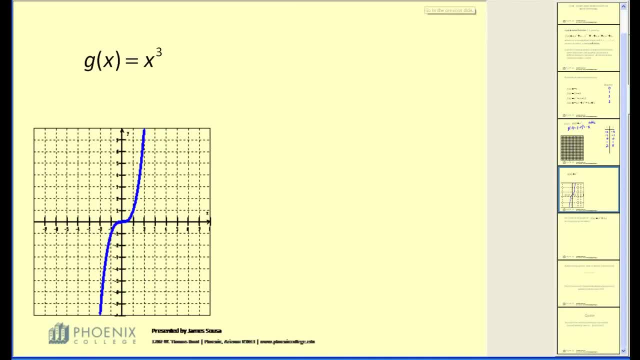 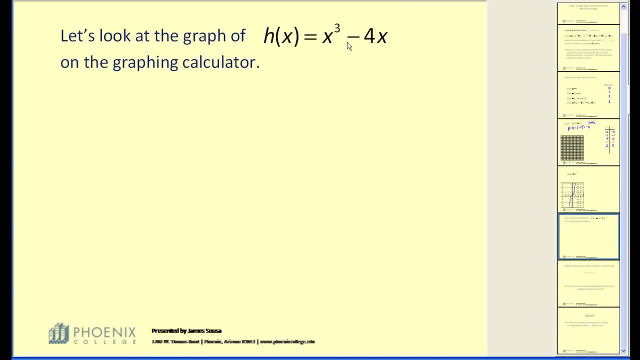 analogy, we will see that it looks like this. So many polynomial functions have curves in it. Let's go ahead and take a look at another cubic function that's a little more involved. h of x equals x cubed minus 4x. By just adding this one extra term, it is going to affect. 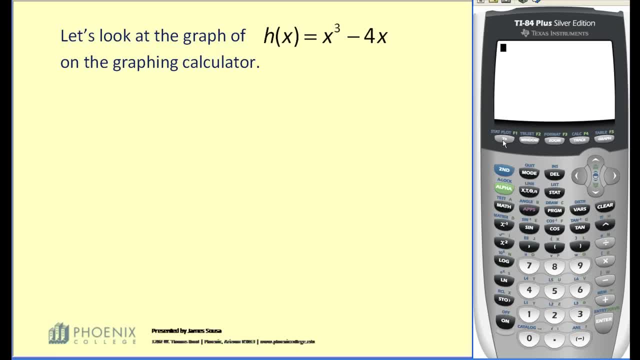 the graph dramatically. Let's go ahead and hit y equals Type in our function x raised to the third power minus 4x. Let's go ahead and hit graph Now, as you can see, just that one term of minus 4x affected. 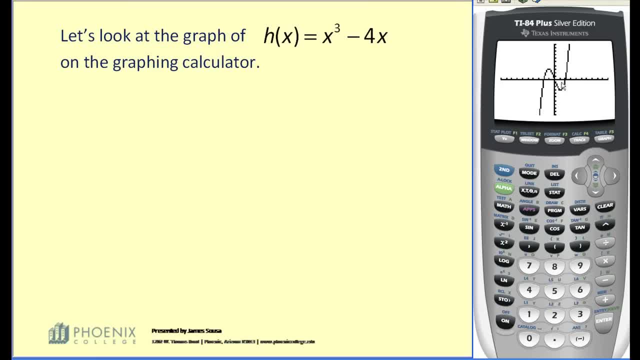 this graph considerably and now has two turns in it And it has a much different shape. So obviously to graph this by hand would take a lot more work. With aid of technology, we can graph this fairly accurately and fairly quickly. If I was to try to graph this on. 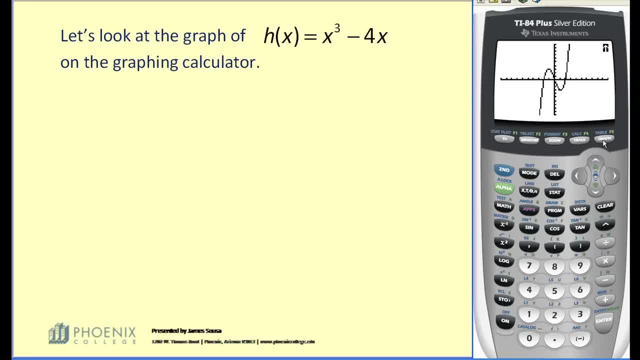 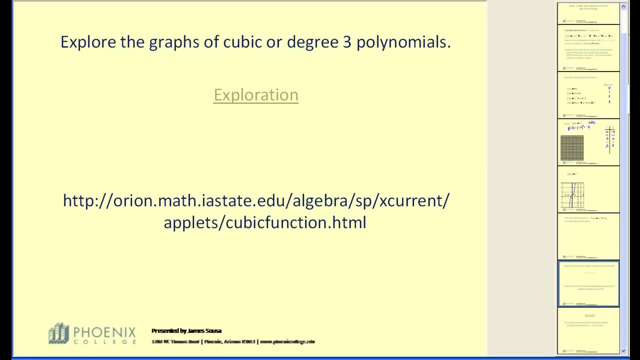 a piece of paper, I would hit second graph and pick several of these points that would be easy to plot and then do the best that I could by hand. Let's explore the graphs of cubics or degree three polynomials. I have a link here to the exploration.